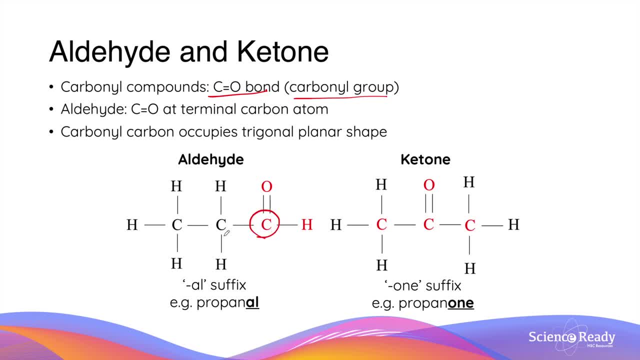 Therefore, the carbonyl carbon is bonded to a carbon atom and a hydrogen atom. In contrast, the carbonyl carbon in a ketone molecule is bonded to two adjacent carbon atoms and no hydrogen atoms. In both functional groups. the carbonyl carbon occupies a trigonal planar shape because it 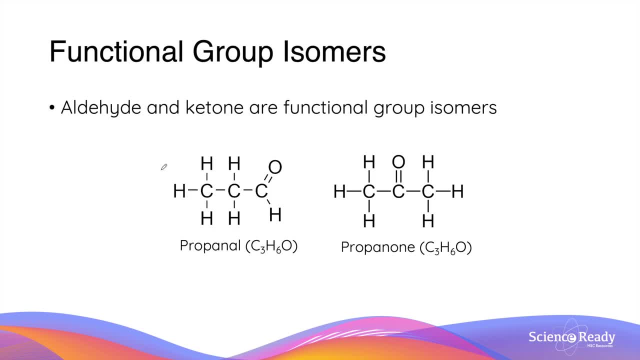 is connected to three other atoms. Not only are they similar: aldehyde and ketone molecules are functional group isomers. Functional group isomers are molecules with the same molecular formula, but different functional groups. For example, propanol and propanone both have the molecular formula of C3H6O. When naming 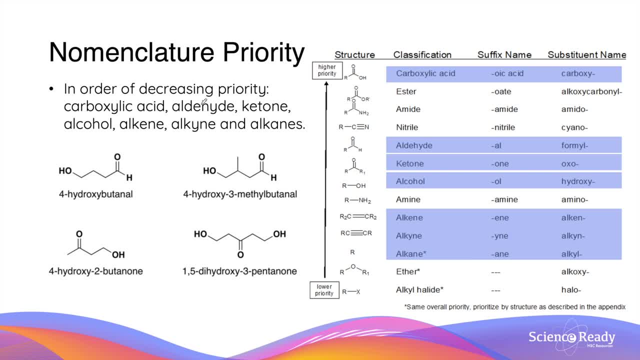 organic compounds. they are called organic compounds. Aldehyde and ketone have higher priority than alcohol and simple hydrocarbons. For example, in a molecule containing both an aldehyde and alcohol functional group, the suffix is Al, which is the aldehyde suffix, while the alcohol is denoted by the prefix. 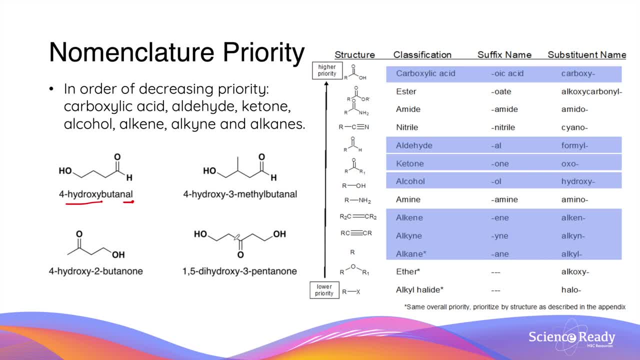 hydroxyl. Similarly, in a molecule containing both alcohol and a ketone, the suffix becomes On for the ketone and On for the propanol molecule. In both functional groups the suffix is Al ketone and the alcohol takes on the prefix hydroxyl. again When analysing boiling point. 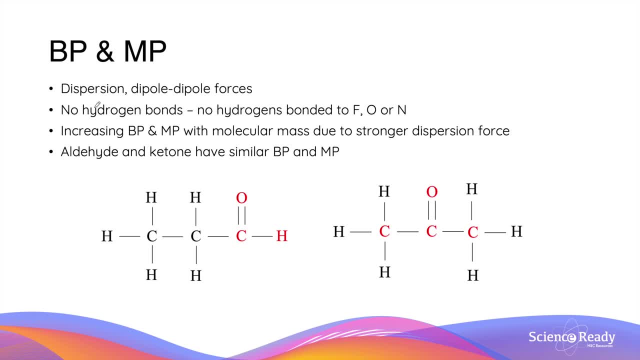 and melting point of aldehyde and ketones, we'll have to examine and analyse their intermolecular forces. Aldehyde and ketones have dispersion and dipole-dipole forces due to their polarity. However, they cannot form hydrogen bonds between the molecules as they do not contain hydrogen. 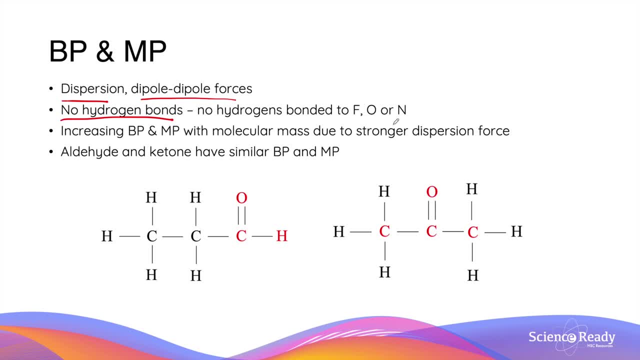 atoms bonded to either fluorine, oxygen or nitrogen. Like every other organic compound, we'll see an increase in boiling point and melting point as the molar mass of the compound increases due to stronger dispersion force. Aldehyde and ketone molecules have similar. 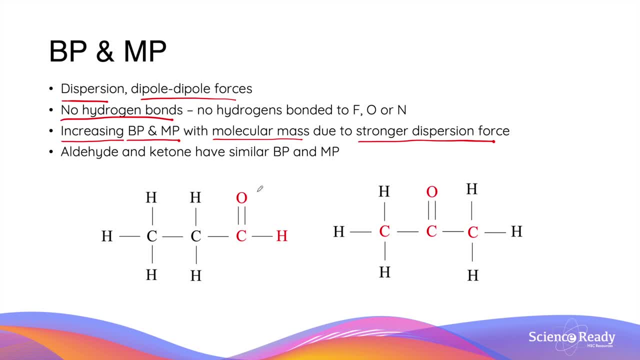 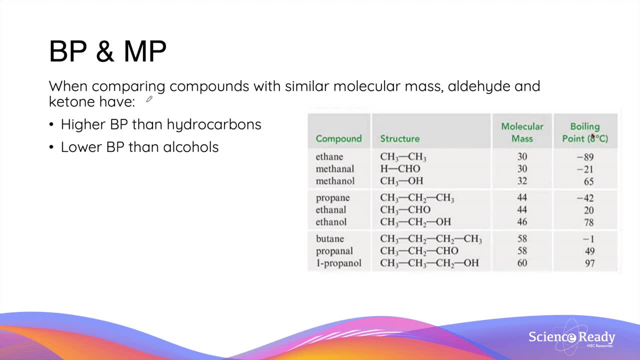 boiling point and melting point due to the similar intermolecular forces they can form between molecules. When we compare aldehyde ketones with hydrocarbons, as well as alcohols of similar molecular mass, the following observations are usually made: Aldehyde and ketones have higher boiling points in hydrocarbons, as hydrocarbons are. 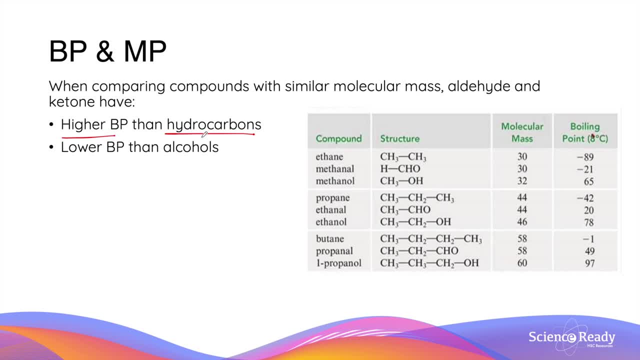 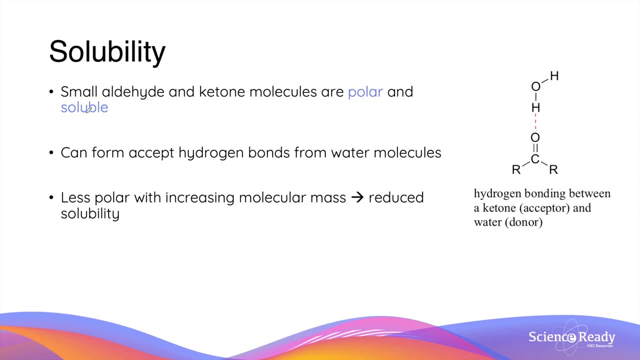 non-polar molecules that are only attracted together by dispersion forces. However, aldehyde and ketones have lower boiling point in alcohols because alcohols can form hydrogen bonds due to the presence of a hydrogen atom bonded to an oxygen atom. 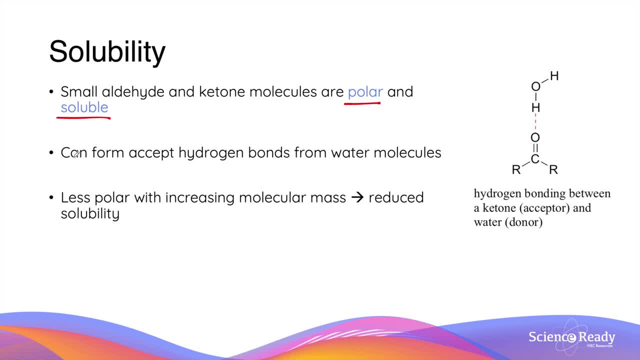 Small aldehyde and ketone molecules are polar and therefore soluble in water. This is because these molecules can accept hydrogen bonds from water molecules. as you can see in this diagram, However, aldehyde and ketone molecules become less polar as the molecular mass increases. 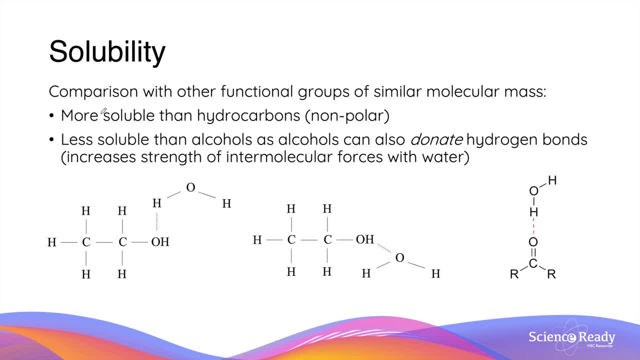 and this leads to a reduced solubility in water. When comparing molecules of similar molecular mass, aldehyde and ketone molecules are more soluble in water than hydrocarbons. Again, this is because hydrocarbons are mostly non-polar. They are, however, less soluble than 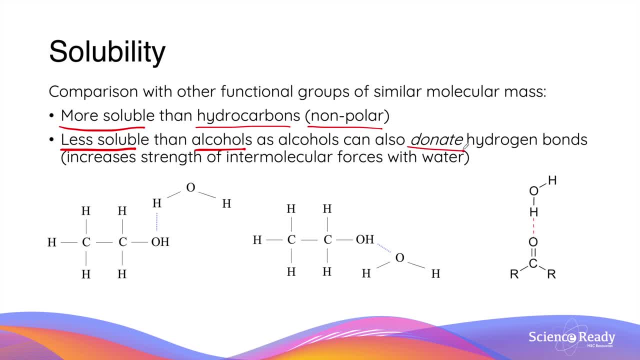 hydrogen bonds, as alcohol molecules can also donate hydrogen bonds as well as accept them from water molecules, This increases the strength of intermolecular forces between the alcohol molecules and water, and thus making them more soluble compared to aldehydes and ketones. 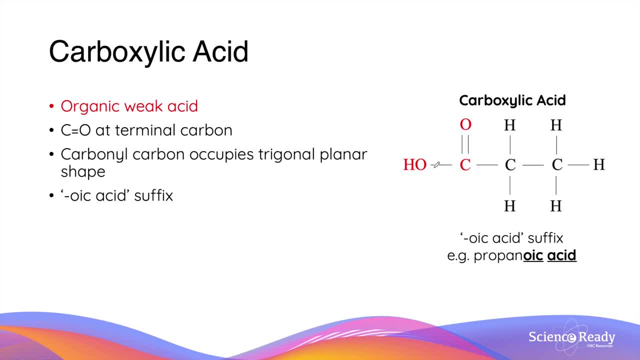 Carbocytic acids are organic weak acids. Structurally speaking, it is a functional group that also contains a carbonyl group, that is, a carbon to an oxygen double bond. Like aldehydes. the carbonyl carbon is located at the terminal end of the molecule bonded. 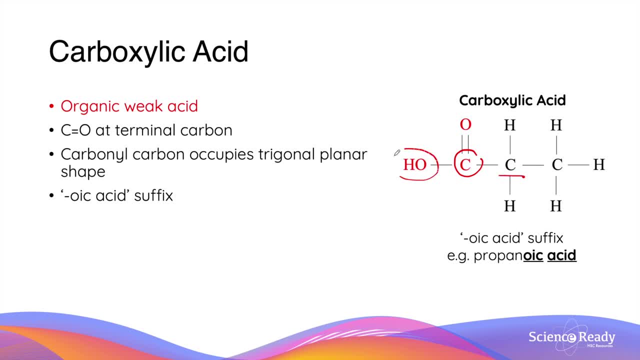 to another carbon atom and, more importantly, an OH group. The carbonyl carbon also occupies a trigonoplanar shape as it is connected to three other atoms. The bond between the oxygen and hydrogen atom in a carbocytic acid functional group is weakened due to the oxygen's 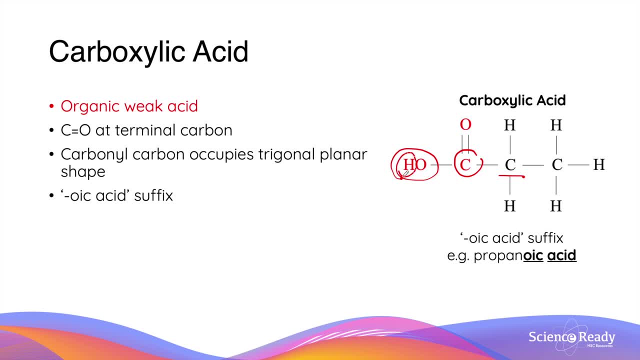 high electronegativity. This enables the hydrogen atom to be deprotonated very easily. When naming carbocytic acids, the suffix "-oic-acid is used. For example, in a molecule with three carbon atoms in the longest chain, the name becomes propanoic acid. 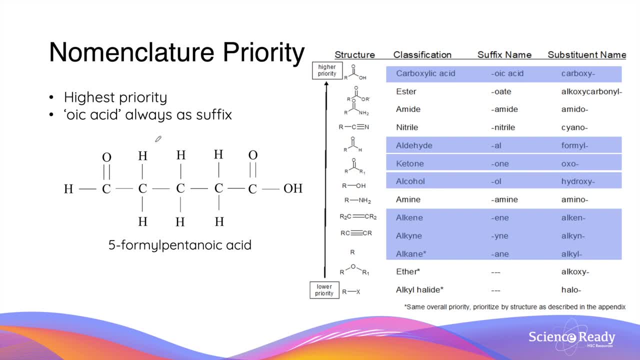 Carbocytic acids have the highest priority when it comes to naming. This means in any molecule containing a carbocytic acid, it will always take the suffix "-oic-acid". For example, in a molecule with an aldehyde and a carbocytic acid functional group, the 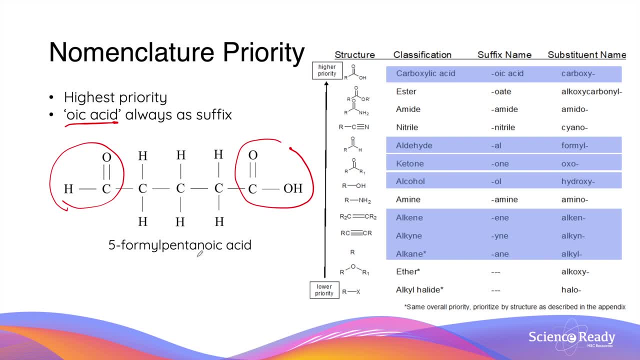 carbocytic acid functional group has higher priority, so it takes the suffix "-oic-acid", while the aldehyde takes the prefix which is formal, so the name becomes 5-formal-pentanoic acid. As mentioned earlier, the main chemical property, 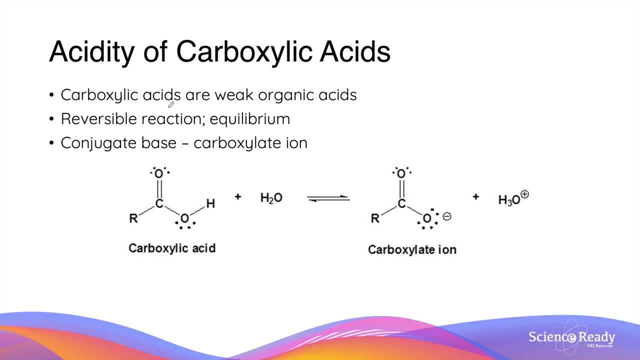 of carbocytic acid is that it is acidic in nature. They are specifically weak acids, so therefore they partially ionise. The ionisation of carbocytic acids are reversible reactions that will exist in a dynamic equilibrium When ionised carbocytic acids will donate. 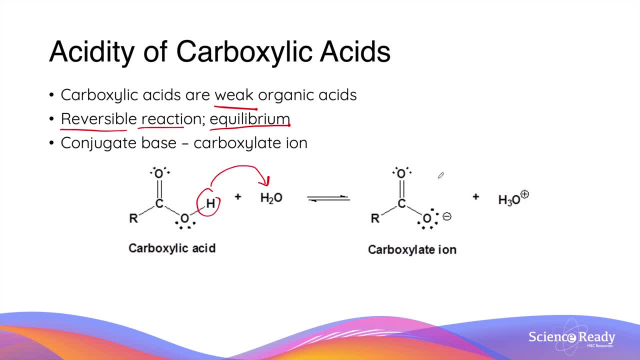 the proton to a water molecule to produce its conjugate base, carboxylate ion, and hence producing a hydranium ion, causing the solution to become acidic. Carbocytic acid molecules can form dispersion forces, dipole and then form an ion. 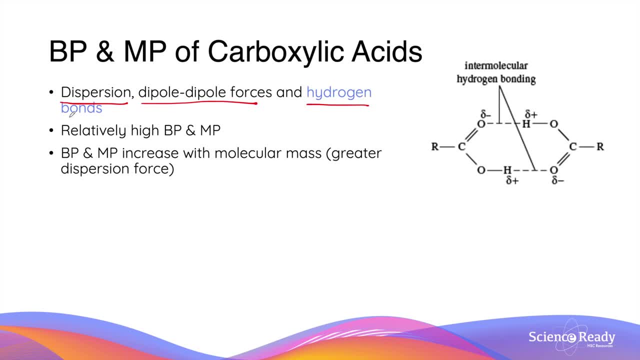 Carbocytic acid molecules can form dipole-dipole forces, as well as hydrogen bonds, due to the presence of a hydrogen atom that's connected to an oxygen atom. Thus they have a relatively high boiling point and melting point when compared to other types of organic functional. 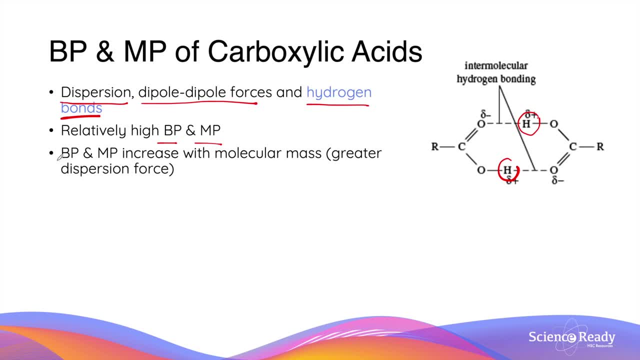 groups. Like every other functional group, however, their boiling point and melting point increases with their molecular mass due to stronger dispersion forces. When compared with other functional groups of similar molecular mass, they have a higher dispersion force as well as a higher boiling point and melting point. Carbocytic acids have higher boiling. 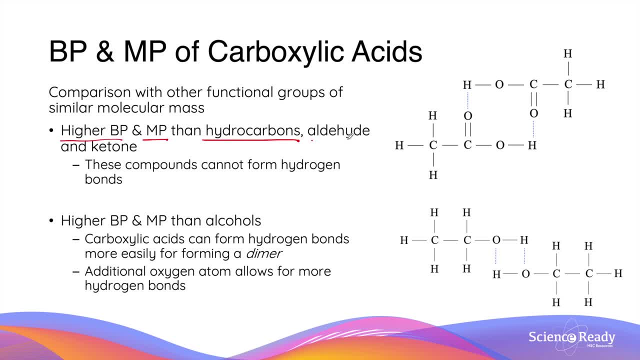 point and melting point than simple hydrocarbons, aldehydes and ketones, as all of these molecules cannot form hydrogen bonds. When we are comparing carbocytic acids with alcohols, they also have higher boiling point and melting point, despite the fact that both alcohols and carbocytic 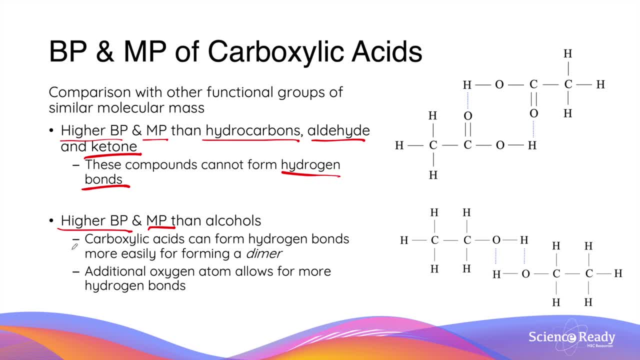 acids can form hydrogen bonds, as you can see here. This is because carbocytic acids can form hydrogen bonds more easily by forming dipole-dipole forces. Carbocytic acids can form more hydrogen bonds by forming this diamond structure, as you can see at the top here. 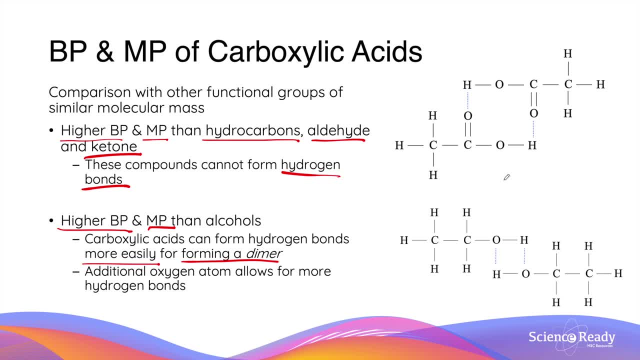 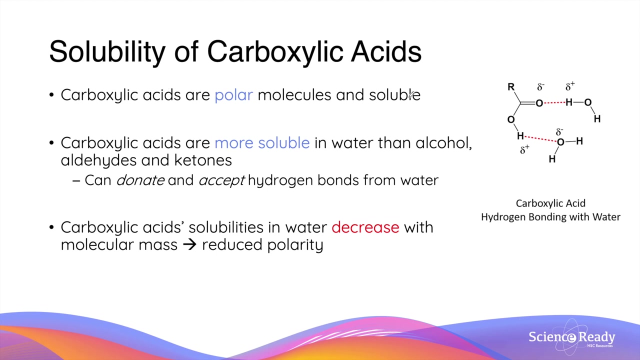 Furthermore, the additional oxygen atom found in the carbocytic acid functional group allows for more hydrogen bonds to be formed. thus, on average, carbocytic acid molecules can form more hydrogen bonds than alcohol molecules can, resulting in a higher boiling point than alcohol molecules. Carbocytic acids are polar molecules and therefore they are 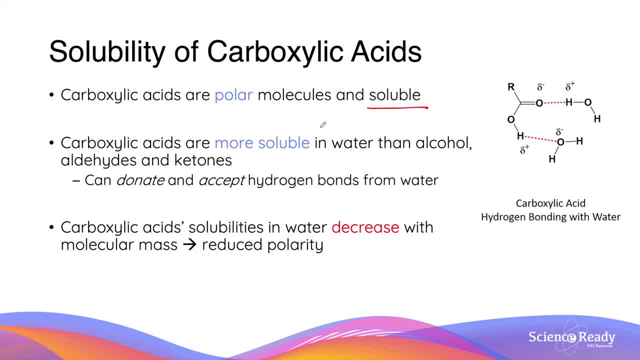 generally soluble in water. They are more soluble in water than alcohols, ketones and aldehydes, as they can both donate and accept hydrogen bonds from water. Like every other compound, carboxylic acid solubilities decrease with the molecular mass due to reduced polarity. 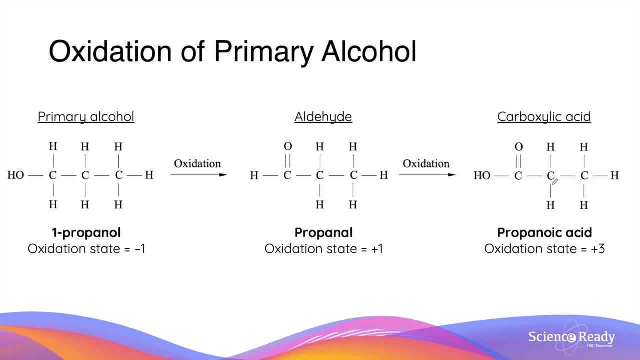 of the molecule. Aldehydes and carboxylic acids can be produced from oxidation of a primary alcohol. Oxidation of a primary alcohol first produces an aldehyde, which is in turn oxidized to produce a carboxylic acid. A weak oxidizing agent such as PCC is used to produce 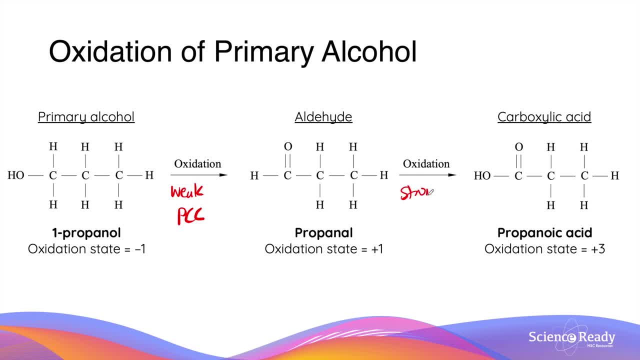 an aldehyde from a primary alcohol. A strong oxidizing agent, such as acidified dichromate ion, is used to further oxidize an aldehyde to produce a carboxylic acid. A ketone-fungible compound can be used to produce an aldehyde from a primary alcohol. 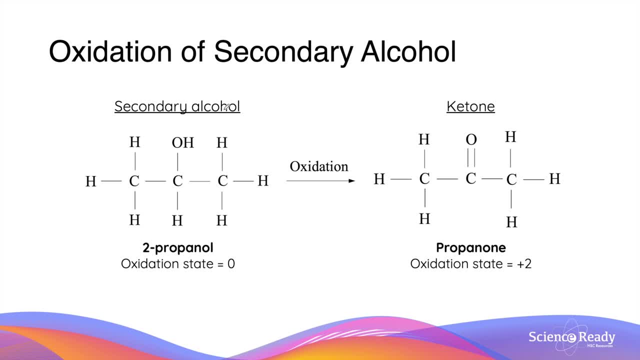 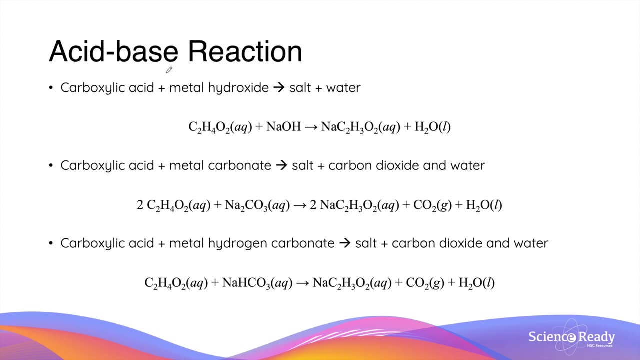 A functional group is produced when we oxidize a secondary alcohol, and this is by using very similar oxidizing agents such as acidified dichromate. Since carboxylic acids are weak organic acids, they can undergo acid-based reactions. So here's a recap of all the important. 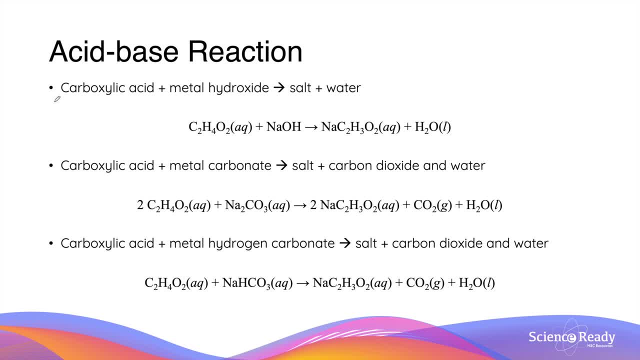 reactions from 1-6: acid-based reactions. Carboxylic acid, when reacting with metal hydroxide, produces salt and water. This is because the metal hydroxide is classified as an Arrhenius base, In this example, ethanoic. 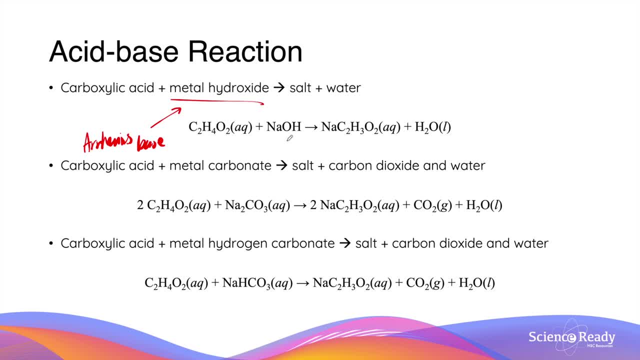 acid. so carboxylic acid with two carbon atoms reacts with sodium hydroxide to give you sodium acetate and water. The second reaction is between a carboxylic acid and metal carbonate, and this produces a salt, carbon dioxide and water.